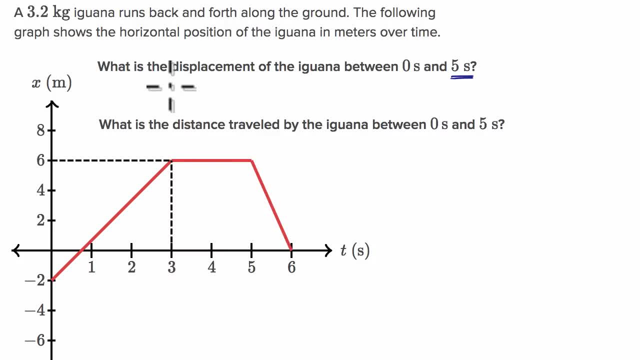 Well, displacement is just your change in position and sign matters. We care about direction, So it's going to be your final position minus your position, Your initial position. Well, what is your final position? Well, we're not talking about the final. 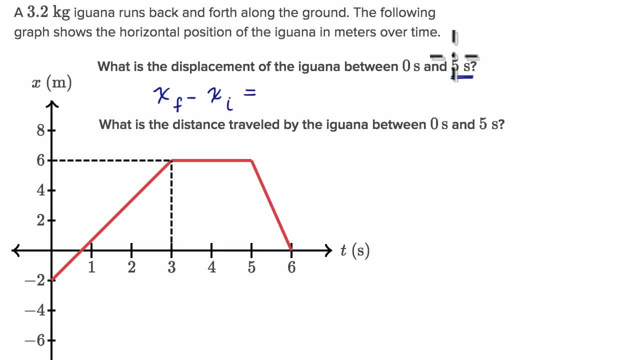 the last time that we have on the graph Here. our final is going to be at five seconds, So our final position is at a positive six meters. So our final position is positive six meters and from that you're going to subtract our initial position. 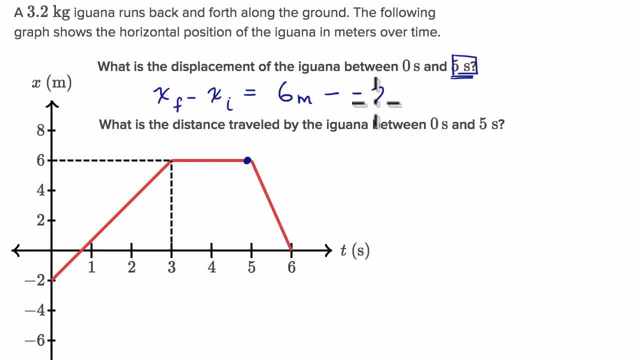 Well, our initial position was at negative two meters, negative two meters, and so this is going to be equal to six minus negative two. Negative two is positive eight meters. So one way to think about it is net. this iguana shifts eight meters in the positive direction. 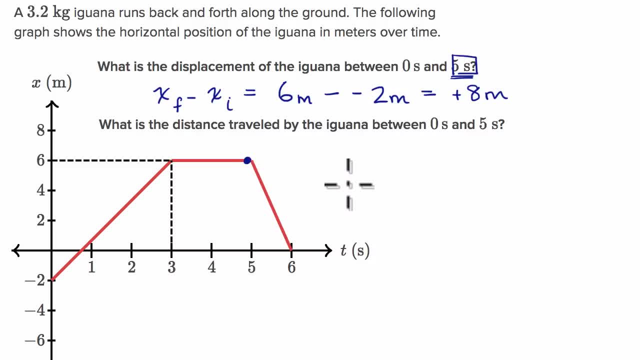 and if we think positive direction is, say, to the right, it would be eight meters to the right. We could draw a number line here. So if we- it's sometimes confusing because we're talking about the horizontal direction but we're plotting position vertically here- 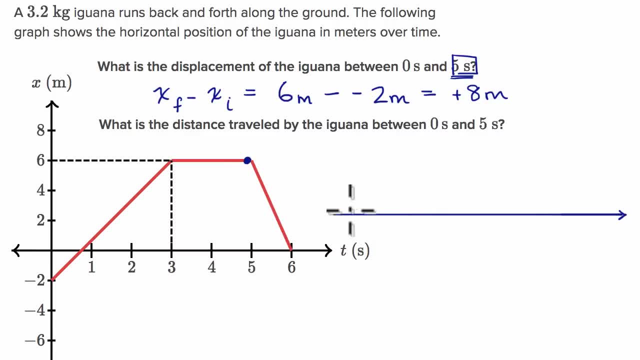 But we could take the same number line and make it horizontal and you'd have negative six, negative four, negative five, Four, negative two, zero, two, four, six, eight. And so what's happening here is the iguana is starting at negative two. 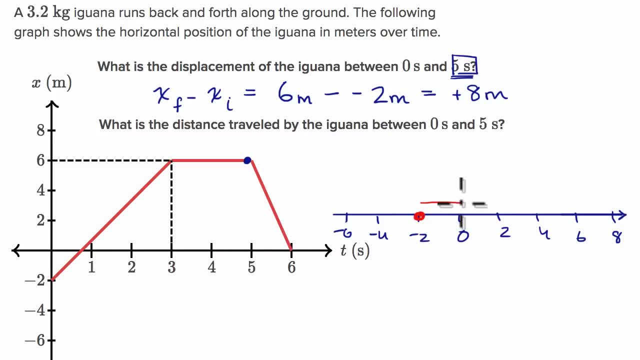 and then, over the next three seconds, it goes to positive six, It goes over here, and so it shifts to the right by eight, and that's what we saw right over there. Six minus negative two is eight. Now what about the distance traveled? 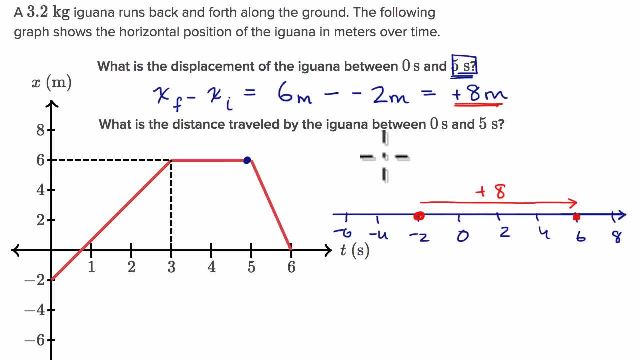 by the iguana over that same time period. Pause the video and see if you can figure it out. Well, the distance is the total length traveled, the total path length. But once again it went from negative two all the way to positive six over the first three seconds. 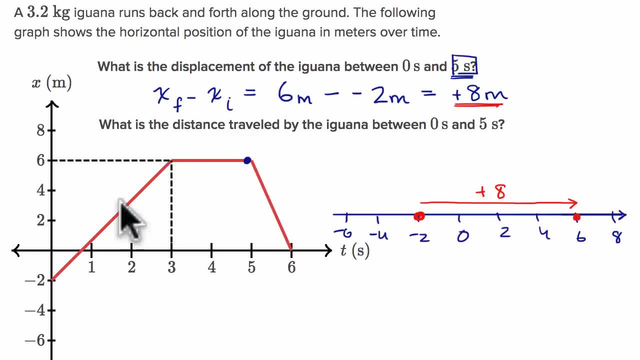 and then it just stays there. So if we think about distance, we're actually going to get the same result. even though we don't care about direction here, we just care about the magnitude, We still get the same thing. It traveled eight meters. 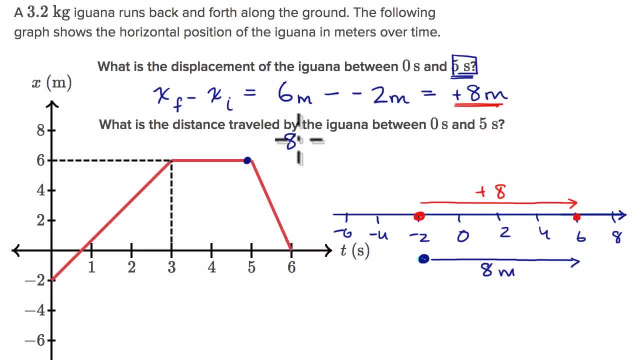 So it travels eight meters. So we're going to get the exact same result. Now, what would be interesting is to think about what would be different if, instead of five seconds, if this said six seconds, If this was between zero and six seconds. 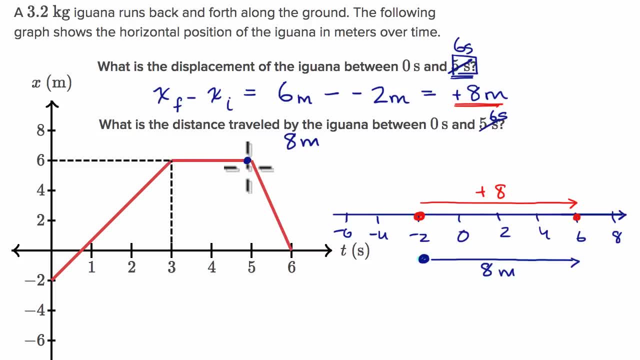 Well then for displacement we would say: hey look, we went plus eight, but then we're gonna go another negative six. So this, right over here, let me make that We're gonna go another negative six And so you actually have. you would have. 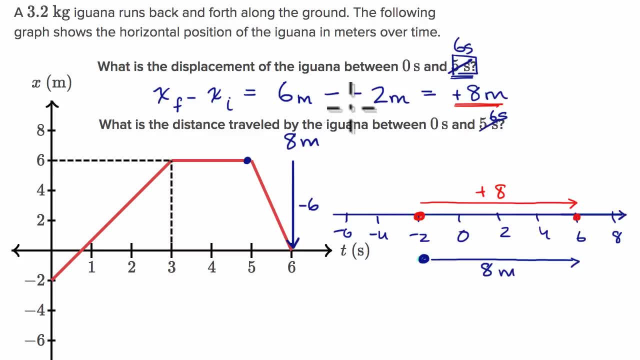 the plus eight minus six. So if you did it for all the way to the sixth second, then your displacement is going to be plus two meters. You have the eight and then you subtract the six. Another way to think about it is you would finish at zero. you started at negative two. 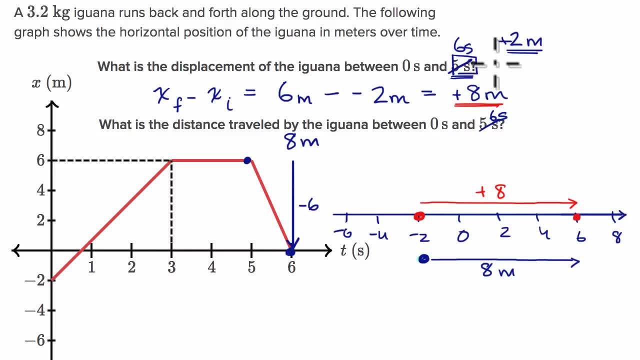 zero minus negative two is two. If you wanted to think about the distance between zero seconds and six seconds, well, you would have this eight meters, and then you would go, even though you're going back to zero. so you're going back to zero right over here. 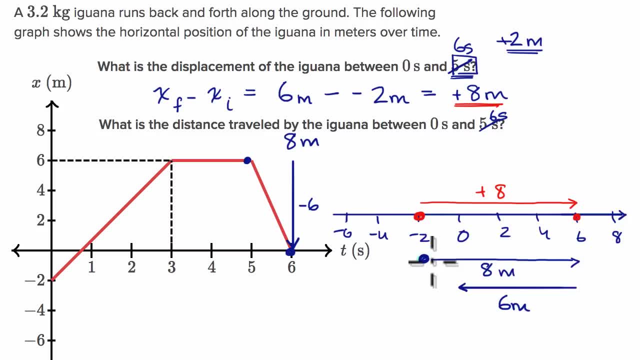 six meters. you wouldn't subtract it because the total path you travel eight meters to the right and then six meters to the left, And so you would add them. So if you said over the first six seconds instead of the first five seconds, this would be 14 meters. 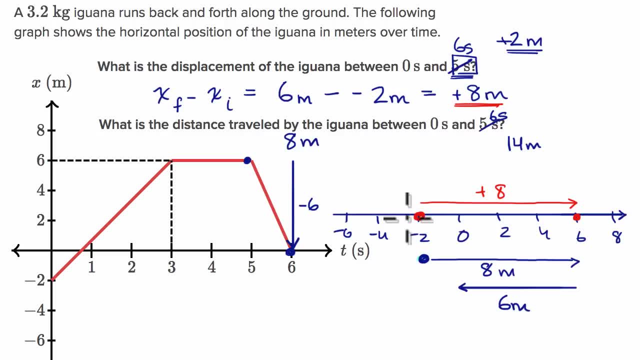 Let me make that clear again: Displacement and distance: in both cases you have plus eight over that first leg, I guess you could say. And then, when we thought about displacement, we subtracted because we're now moving to the left. 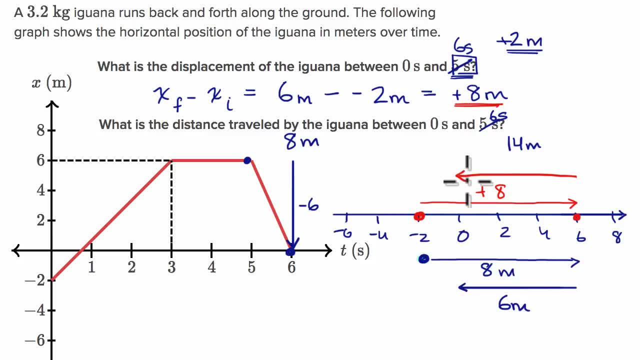 we move to the left by six. So in the case of displacement, you subtract the six and you have a net displacement of plus two. But distance, the total path traveled, you have the eight to the right and then six to the left. 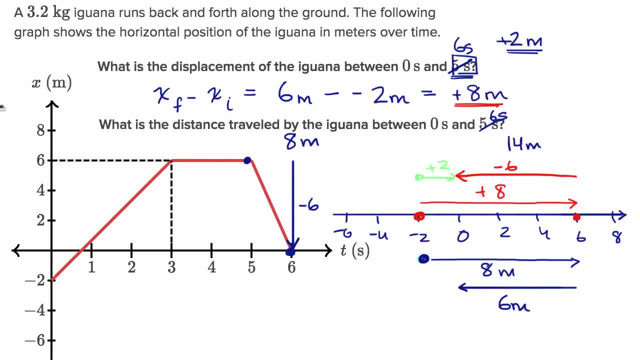 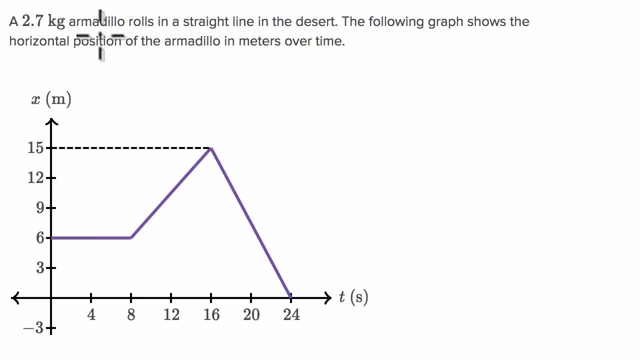 which gives you a total path traveled of 14.. Let's do one more example here. A 2.7-kilogram armadillo rolls in a straight line in the desert. The following graph shows the horizontal position of the armadillo in meters over time. 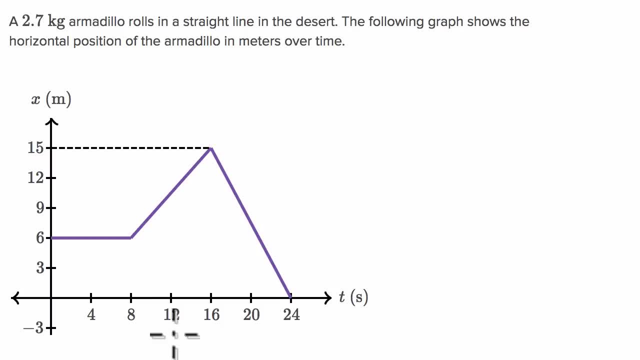 And so let's think about the same thing Over the first 24 seconds. let's go all the way to the 24th second. let's think about what the displacement is and what the distance traveled is. So first pause this video and see if you can figure out. 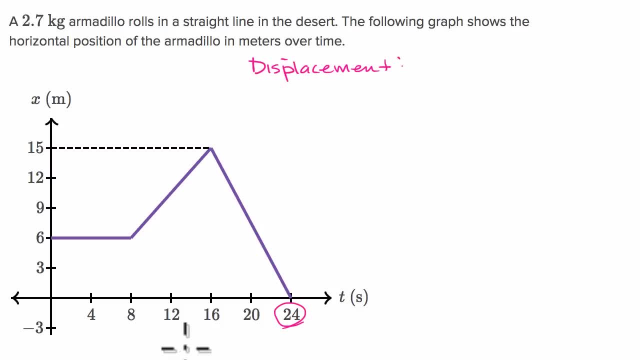 the displacement. What is the distance traveled over the first 24 seconds? Well, this is going to be our final position minus our starting position. Our final position: we're at zero meters. Our starting position: we were at time zero. we were at six meters. 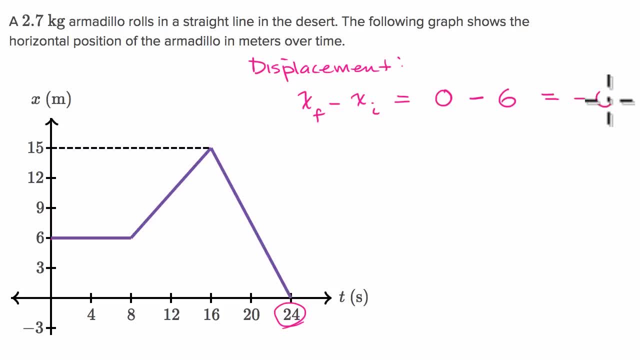 All right, let me just write the numbers down. So it is negative six. Let me say that one more time At time 24, notice our vertical coordinate. We are at a position of zero. That's where that came from When we started, at time zero. 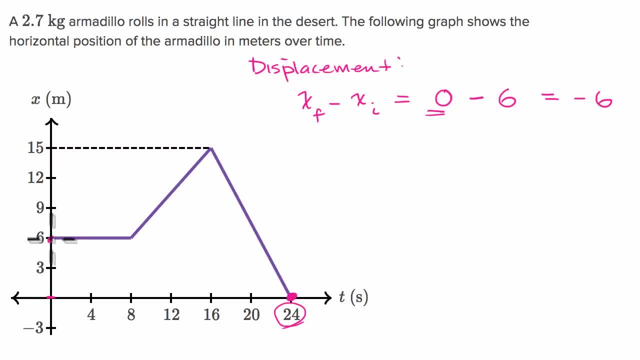 our position was right over here. So our final minus, our starting, is negative six, And you could also see that If you just look along this line, we shifted from positive six to zero, which would be a shift of six to the left if you made this horizontal. 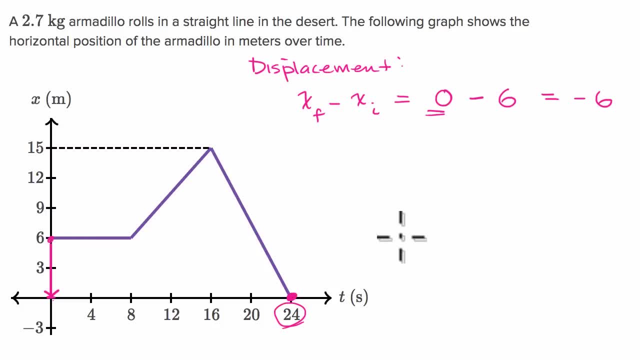 or a displacement of negative six. Let me draw this on a horizontal line just to make this a little bit clearer. All right, Let's make this a little bit more clear. So, if you have zero four, oh, zero three, six, nine, 12,, 15, so on and so forth, 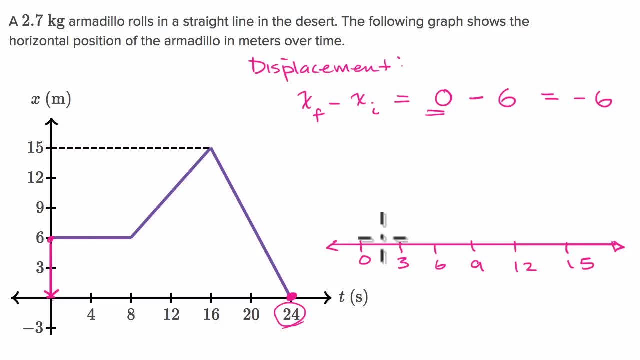 we are starting at six. Let me do that purple color. We're starting at six. We do a bunch of stuff in between, but then we end up after 24 seconds at zero. So our shift. we went six to the left. 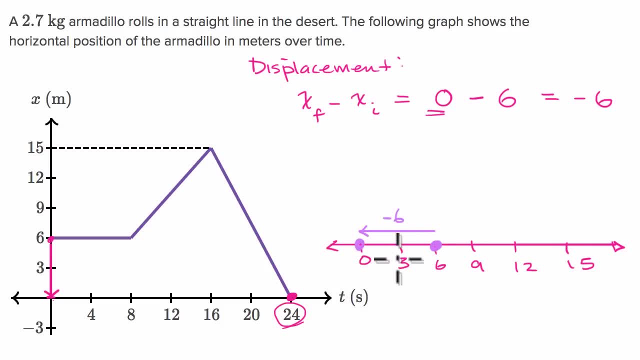 or we have a displacement of negative six. Zero minus six is negative six. So now let's try to figure out distance. Pause the video and figure out the distance that this armadillo travels over this 24 seconds. So this is interesting. 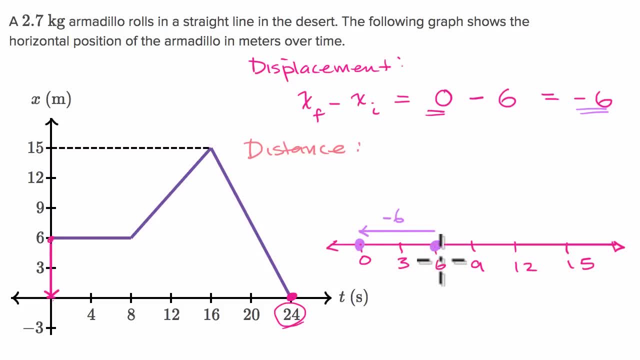 So it's right here. It starts off at position of six. So let me do it right here. It starts off at position of six. It stays there. It stays there for the first eight seconds, Then from the eighth second to the 16th second. 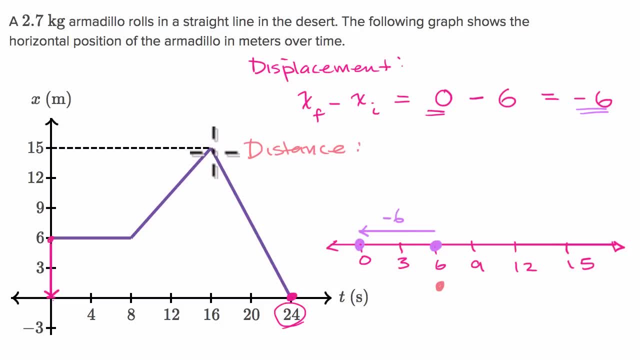 its position increases by nine to get to 15.. So it does this, It goes to 15.. So this is going to be plus, this is going to be plus nine, And then, on the 16th second, it goes from 15 back to zero. 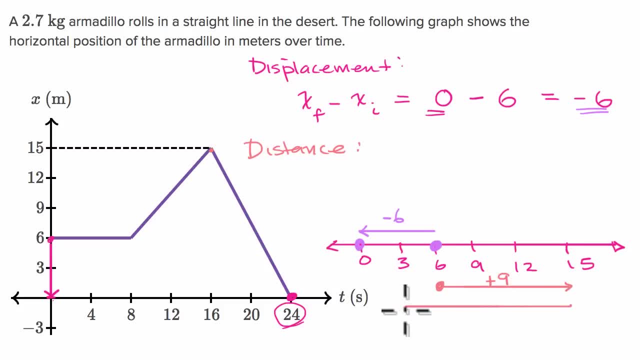 So it goes from 15 back to zero. So it goes from 15 back to zero. So it goes from 15 back to zero. If we were thinking about displacement, we would write a minus 15 here and then we would net these out to get to a negative six. 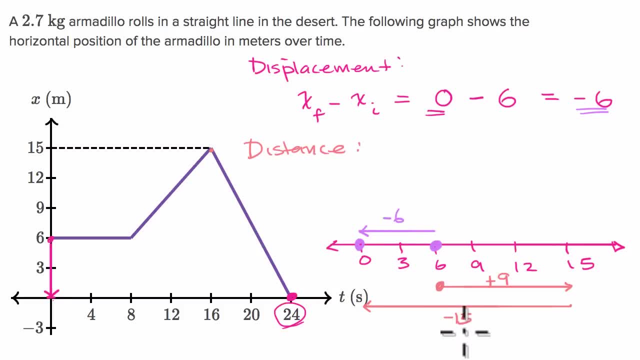 But we're thinking about distance, So we think about the absolute value of the various parts of the path traveled. So all of these are gonna be positive. We just say, hey, what is the total journey? So this is going to be plus 15.. 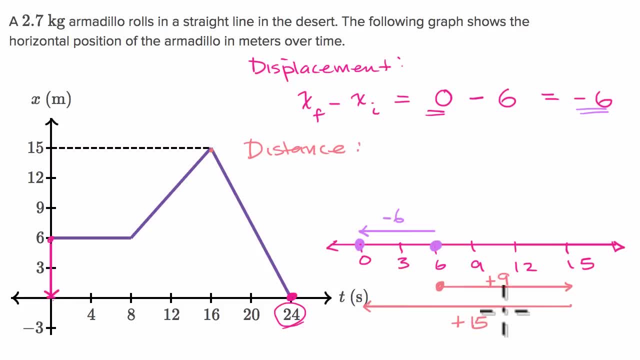 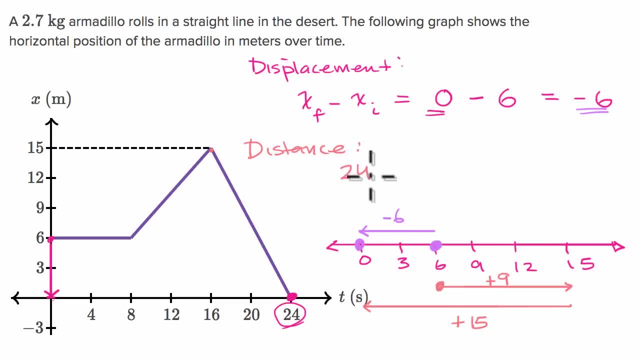 So this is interesting: Even though the armadillo traveled a total of 24 meters, its entire path was 24 meters long. its net shift, its displacement, is six meters to the left, And this is another thing to emphasize This negative number. this is implying direction. 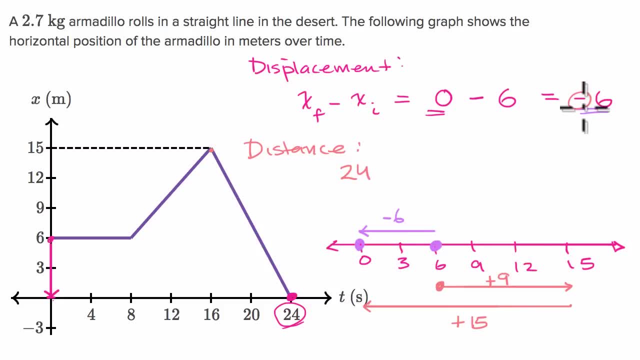 It's saying: if we look at this number line, it's saying to the left, Even if it was a positive six, because we're talking about displacement, it would imply positive would mean to the right Distance. doesn't tell you about direction. 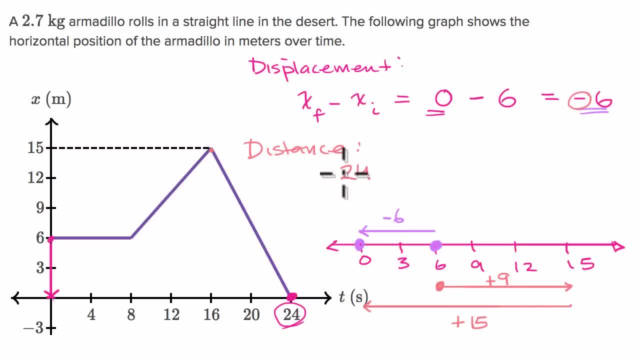 It just tells you the absolute magnitude of the total distance traveled or the length of the path.